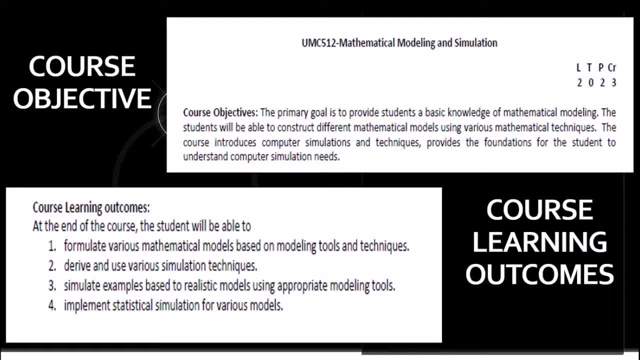 simulations and techniques provides the foundations for the student to understand computer simulation needs. So, as you can see, the name of the course is mathematical modeling and simulation. so it's not only about theoretically, construction of mathematical models, it's also about learning various simulation techniques. and this is the area of simulations are also performed on computers. so 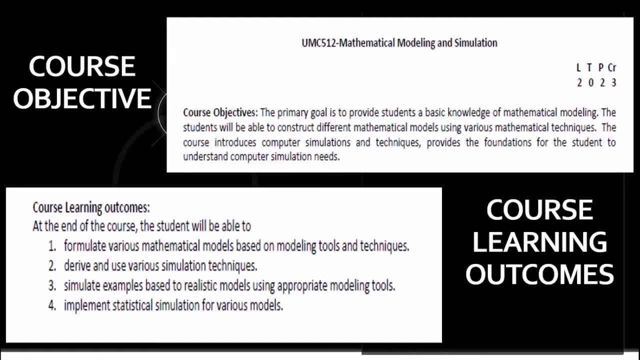 specifically, they are computer simulations, so they are not limited to the numerical techniques. simulation is a much general word. so all of these things you will learn in this course and you will be able to create your own simulation techniques. So this is a very important point about. 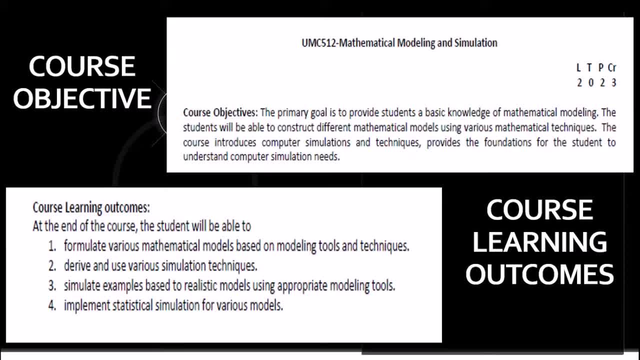 simulations for different models and if you look at the course learning outcomes, so you can read at the end of the course- the student will be able to formulate various mathematical models based on modeling tools and techniques. so this is one of the objectives. so obviously we want this to be. 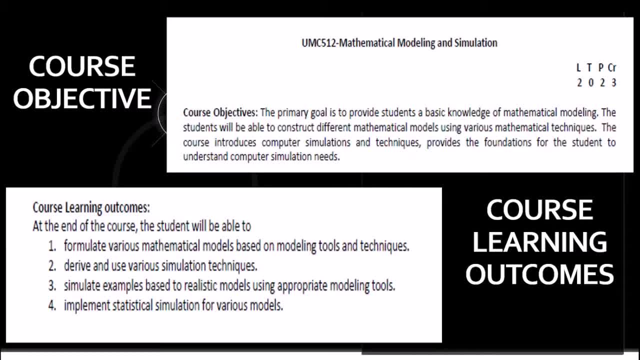 fulfilled that once you complete this course. so you should be confident in formulating various mathematical models yourself, Derive and use various simulation techniques- so this will also be learned- and simulate examples based on realistic models using appropriate modeling tools. so, as I just told you, the simulation will vary. the type of simulation will vary according to model to model. so we have to 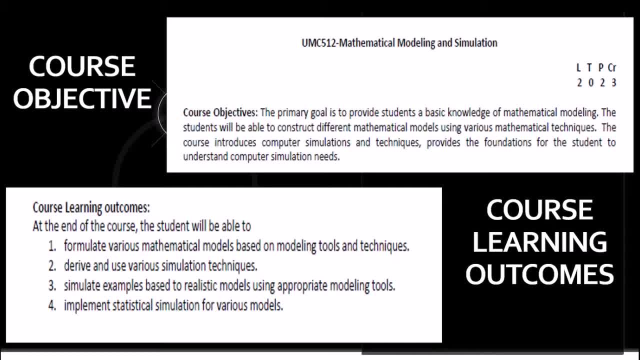 develop the simulations depending upon what particular appropriate model we are focusing on. so this you will also learn: Implement statistical simulation for various models. so so far, you might have studied the course of probability and statistics. so whenever, in this course particularly, we'll be talking about the stochastic and statistical models, 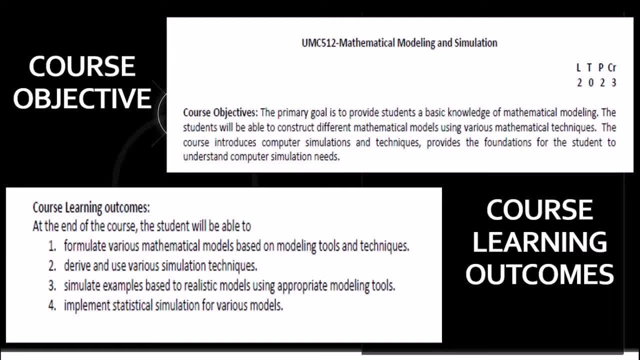 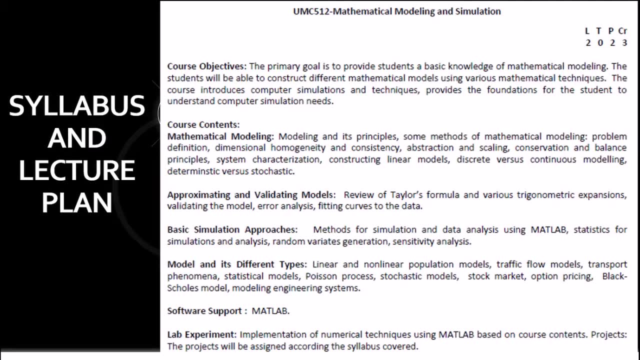 so they're the kind of simulations which you will be doing are coming in the category of statistical simulation, so that also will be one of the course learning outcomes. so let's move ahead to the syllabus and lecture plan. so if you look at the course content, it has been divided in four sections. 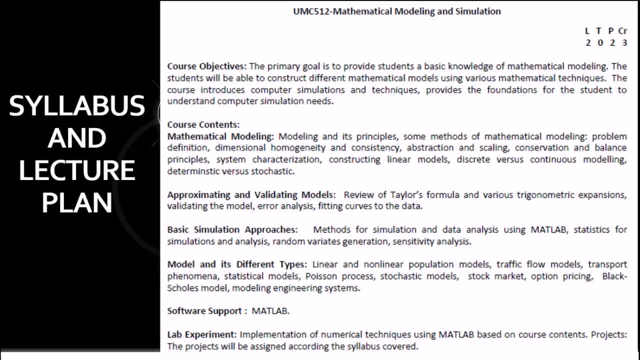 first section is mathematical modeling, which has the components modeling at its principles, some methods of mathematical modeling: problem definition, dimensional homogeneity and consistency, abstraction and scaling, conservation and balance principles, system characterization, constructing linear models, discrete versus continuous modeling and deterministic versus stochastic. so this part, I will say, is a bit theoretical, although the kind of examples we will 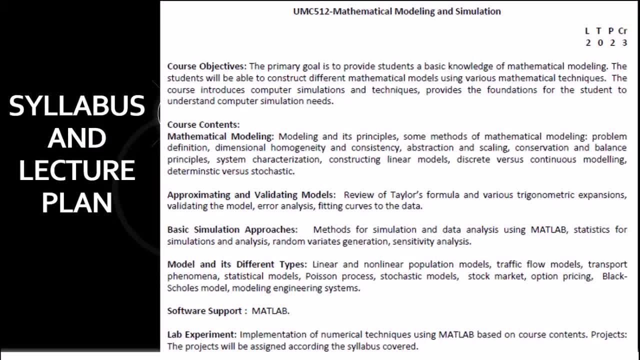 associate with each theoretical concept are going to be engineering applied examples. they are the real-world problems. but this is comparatively more theoretical as compared to the rest of the portion of the syllabus. so the last part, which says discrete versus continuous and deterministic versus stochastic, so that is about the classification of 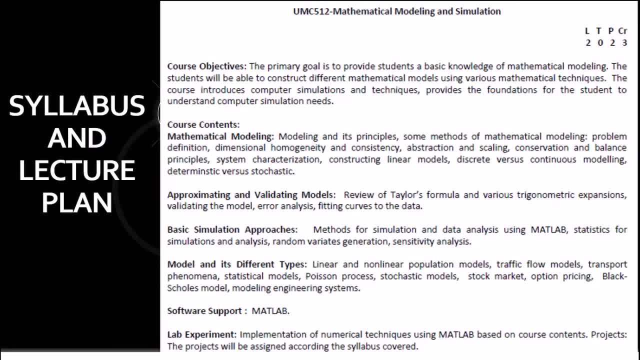 mathematics models, approximating and validating models. so in this we will be reviewing the Taylor's formula and various trigonometric expansions, validating the model, error analysis and fitting curves to the data. so basically, in this you will know something which you already know. you will know that in more detail. 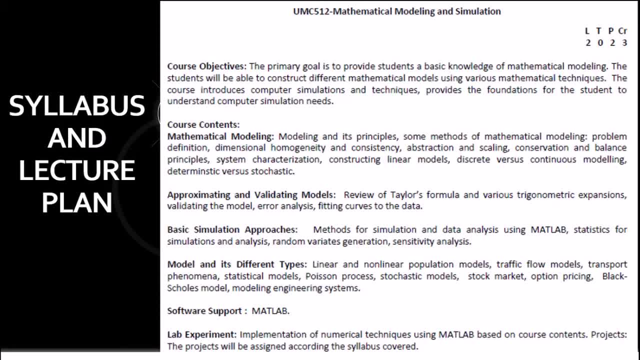 we are already familiar with the Taylor series and its usage in approximation of different trigonometric functions, not only trigonometric functions but also trigonometric functions. but we know there are some specific conditions for a function to satisfy. it can be expanded as Taylor series, so that part we will be 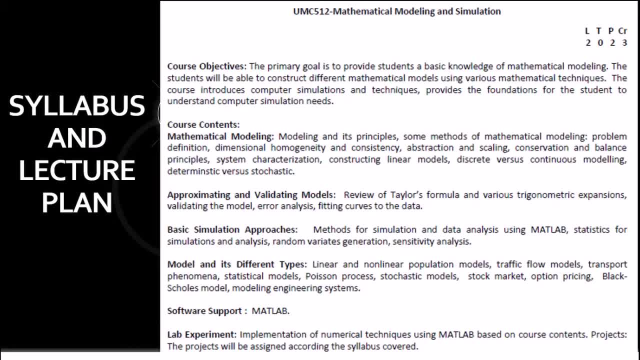 focusing on- and that is something you have already done- validation of model: how, when you construct a model, how it is going to be validated through error analysis and curve fitting. so these are the techniques which you will be learning, and some of this you are already familiar with. so this is majorly the lab part. we will learn this in the next video. 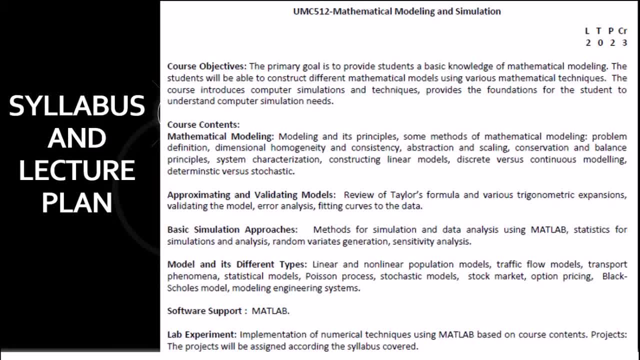 and then we have basic simulation approaches, so methods for simulation and data analysis using MATLAB. so it's clear from here that we will be using MATLAB to do the computer simulations, statistics for simulation and analysis. that is also the component to be covered in lab: random variate generation. so 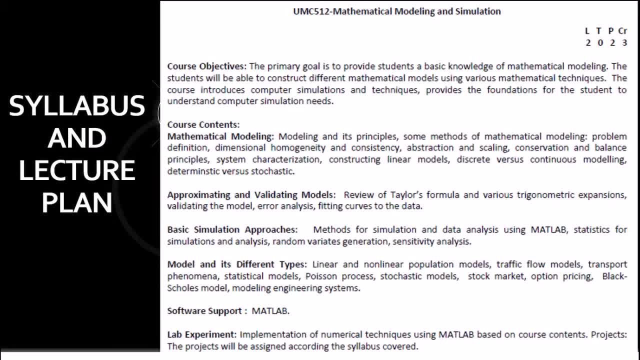 random variate generation is something we will be doing theoretically first and then we will be doing that in lab sensitivity analysis. so sensitivity analysis- you might be familiar with this for the subject optimization techniques, where you have performed sensitivity analysis for different linear programming problems, but here it will be used in a general sense. and the last section, if you look. 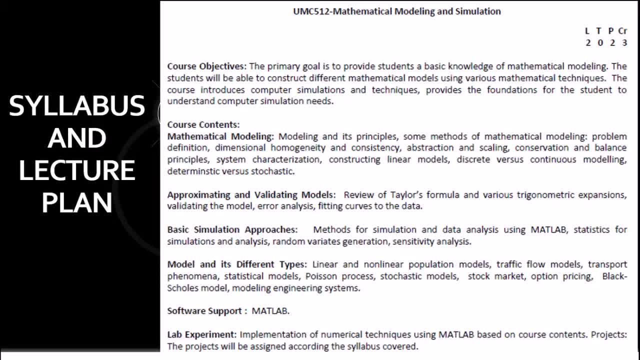 at is actually the most important part: model and its different types. so in this section we have different, different types of models. it's something like the particular examples of mathematical models which we will be taking up in this course. the very first is linear and nonlinear population models. then we have traffic. 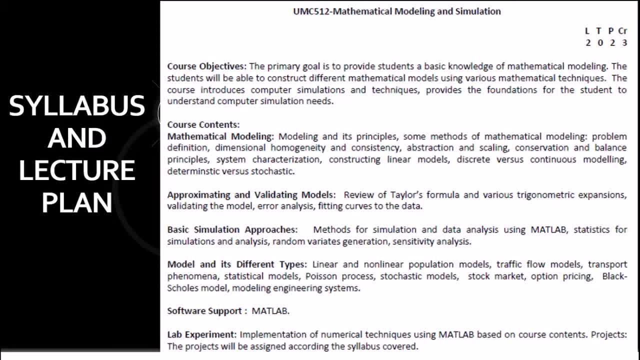 flow models, transport phenomena, statistical models and in statistical models specifically, we have Poisson process, Markov chain and other stochastic models, stock market option pricing, Black-Scholes model. so this this portion- stock market option pricing and Black-Scholes model- this is one part of of introduction to the financial mathematics and because that 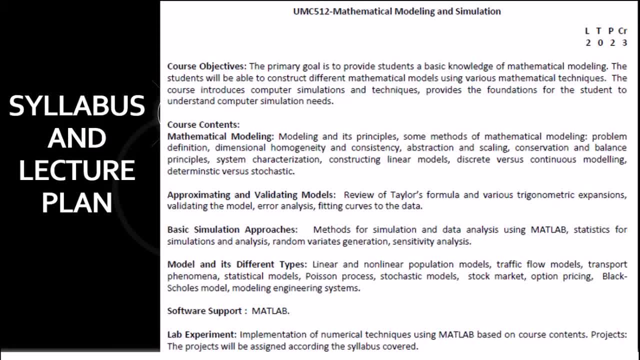 is also one of the course in black-scholes model, so this is one part of of introduction to the financial mathematics and because that is also one of the course in this basket- mathematics and computing- so this knowledge will build up a bridge from this course to the next course, so you will have a fairly good idea about. 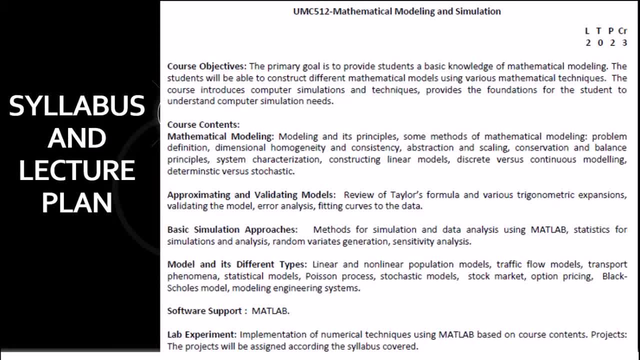 financial mathematics in this course also, and obviously in the next course you will be studying that in more detail. and last but not the least, we have modeling engineering systems. so these examples are spread ever every radio. so now if you talk about lecture plan, so what I would say we will not be covering- teaching in black-scholes with L2 as a глав 실枠. we will not be covering it life to life in the next class. also last, but neither way, unless we will talk or being easy, era FOOOO. so now, if you talk about lecture plan, so what? I would say we will not be covering it life to life. in the next class we would be doing this math, math along your way, which I have shown. 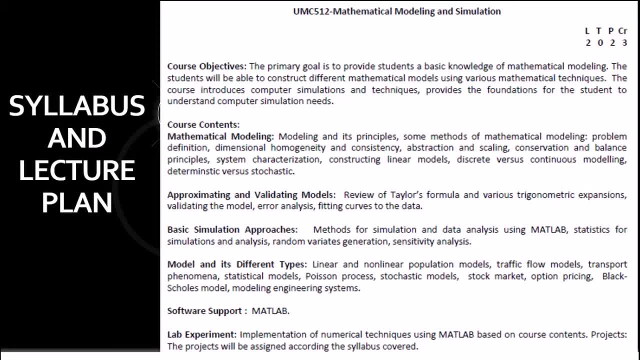 that firstly we have to finish all the theory and then only we will be moving to the specific model examples. we have to maintain a balance of it, because if we first run after finishing the complete theory, then we will not be having anything to discuss in lab simultaneously, because every week we 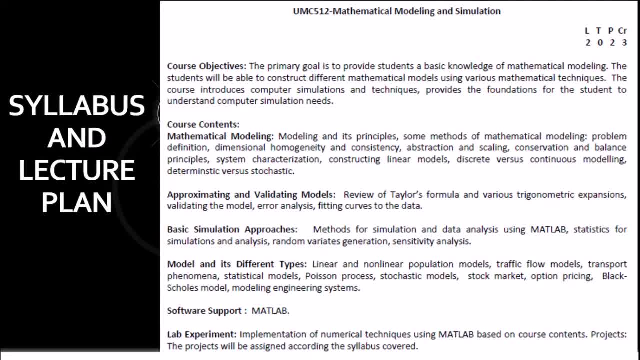 have a lab, so we should have some practical example of particular model so that that can be solved in lab. so what we will do: we'll study some theoretical part and then we'll do some specific model. we'll again continue with the theory and then again some specific model. so this way we'll maintain a 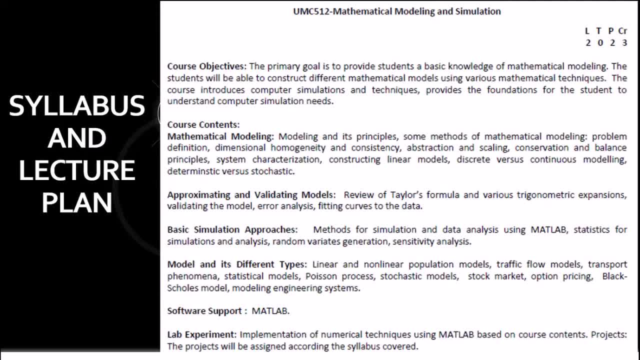 balance. so that's how the lecture plan will be executed and the portion which has to be exclusively covered in lab, so that will go to the lab part. so software support: we are going to use a MATLAB extensively for this and all the lab experiments we'll be doing in MATLAB. 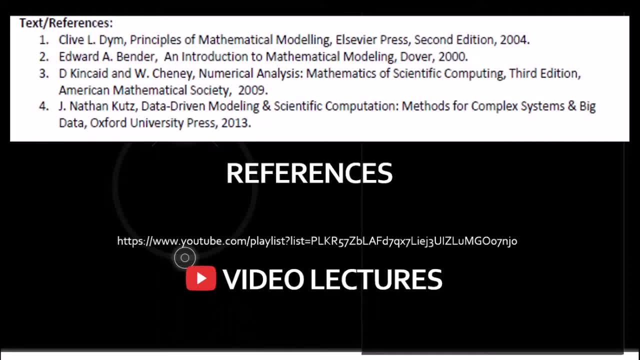 so these are the references and textbooks. so the first book is a very simple and easy to understand book. it's the principles of mathematical modeling, Clive L Dyne. it's a very basic book, and the next book is Edward A Bender, an introduction to mathematical modeling. so the kind of study material or the 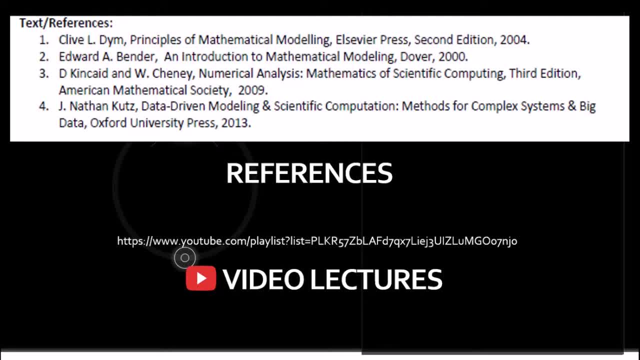 lecture notes which I will be providing to you in the next lecture will be: you is going to be a combination of these two books, the examples taken from one and two, and I will be giving you the assignments which will cover the unsolved questions of these books. also, third and fourth, references are not. 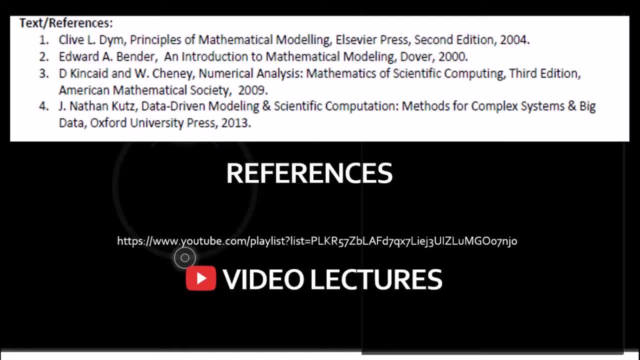 required. these are not mandatory because they are for the numerical part, numerical analysis, and you already are familiar with the numerical techniques. so, depending upon our requirement, will study the numerical technique otherwise for understanding of mathematical formulas. so these are the two books, in a combination of these two books. 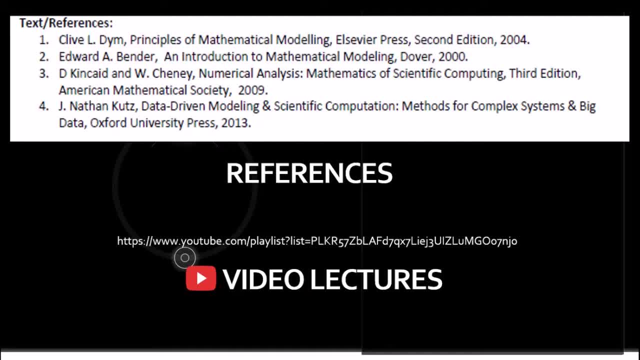 mathematical modeling. we do not require this, at least the third reference. the fourth one is data driven modeling and science, free competition. so that is also an advanced level book. so we may or may not need it and, apart from this, all the video lectures will be available on this youtube link. 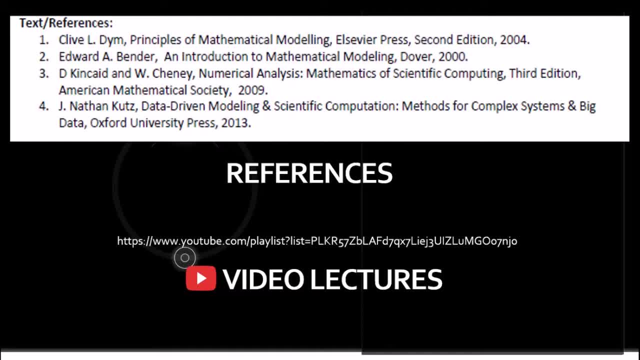 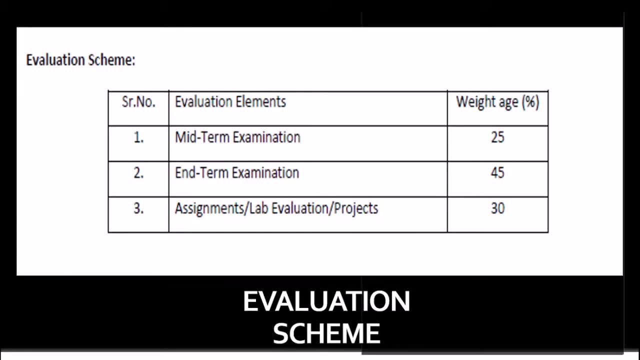 which i will be sharing with you, and every recorded lecture will also be available on the lms portal. if you talk about evaluation scheme, so we'll have three evaluations: midterm examination, end term examination- so the weightage of midterm is 25 percent and term is 45 percent, and the 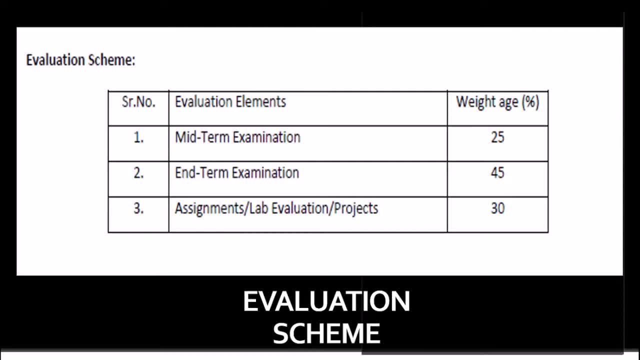 assignments, lab evaluation projects, collectively is 30 percent. so we are not going to comment anything about midterm and end term because that's obvious. we are not going to have any different kind of change there, but these 30 percent which is in the third section, so that we can customize. so i have assigned 15 marks for the 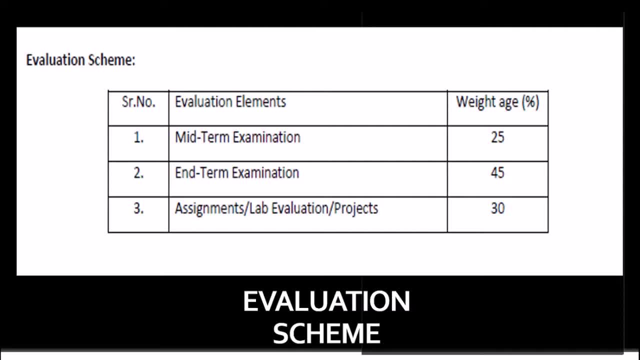 final lab evaluation and 15 marks will be for the project. i will be definitely giving you the assignments, but those assignments will be just to give you an idea about the practice, practice questions, because we do not have a tutorial component, so we cannot have the practice of more. 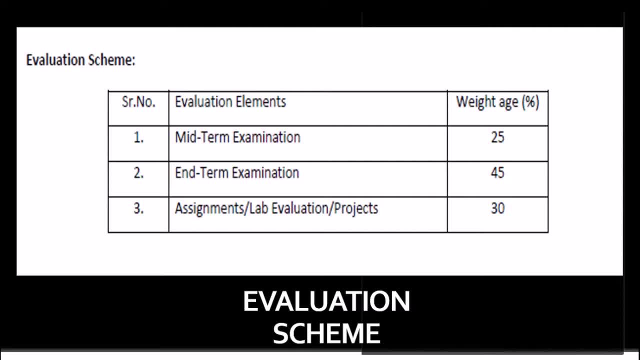 number of questions. so i'll be giving you assignments in that you will be having the questions to practice at home and we can discuss them in either the labs session or some doubt session we can have. but as such we won't be evaluating any assignment, right? so the 15 marks. 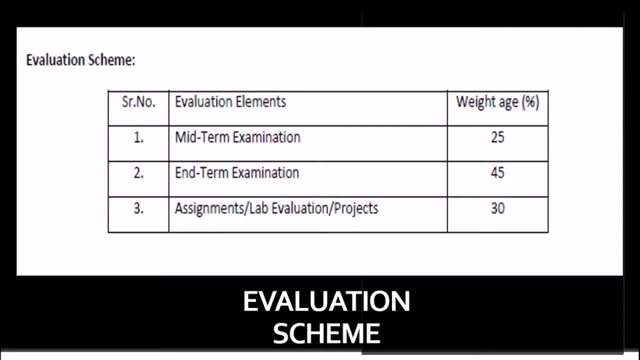 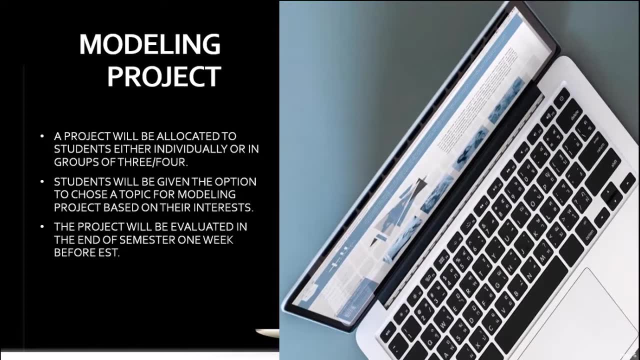 will be for the final lab evaluation, which will be conducted, uh, near the end of the semester, and 15 marks will be for project. so this project will be allocated to you. so let's talk about this. this project is going to be a mathematical modeling project, so a project. 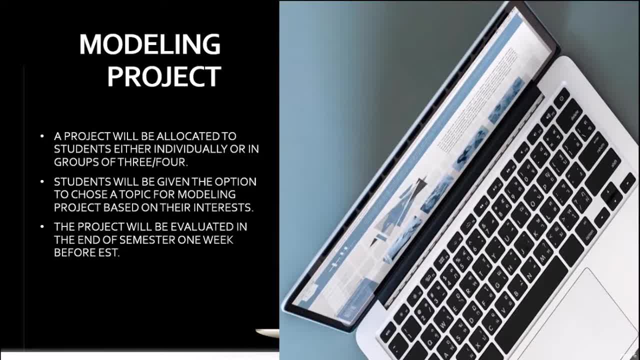 will be allocated to the students either individually or in groups of three to four, so depending upon how we get along with the course, so this thing can be sorted out, that, whether we want individual projects or we want to combine the groups, right, because all of you are at your homes studying online, so, uh, it might not be possible to form groups physically, so it 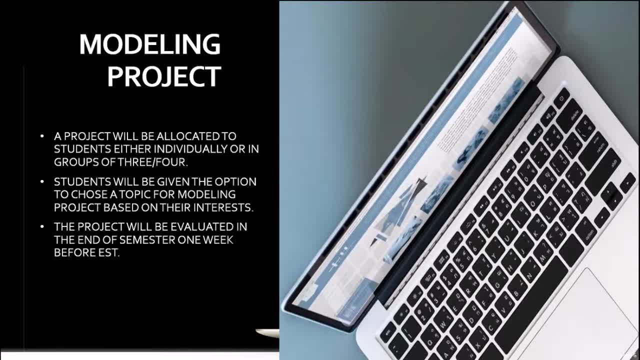 might be possible that we can work individually on certain projects. so the projects will be given to you on a topic of your choice, based on your interest. so you will be given a selection of topics and from there you figure out one option and i will try my best to allocate you the project. 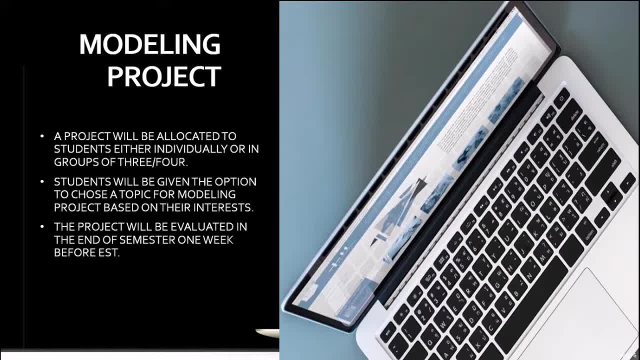 according to your interest and the project will be evaluated in the end of the semester, one week before asd. that will be the final project evaluation, but in between also we'll have something about the project. that evaluation that will not be a formal evaluation but that will be a kind of a. 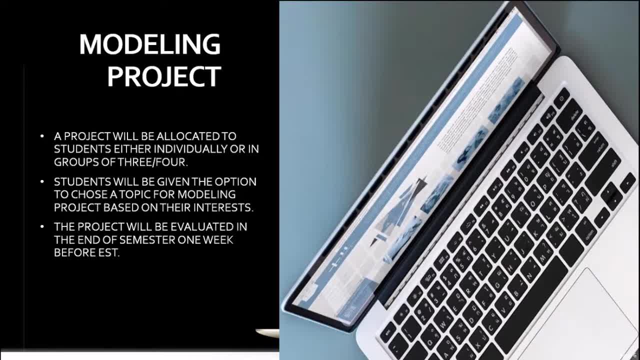 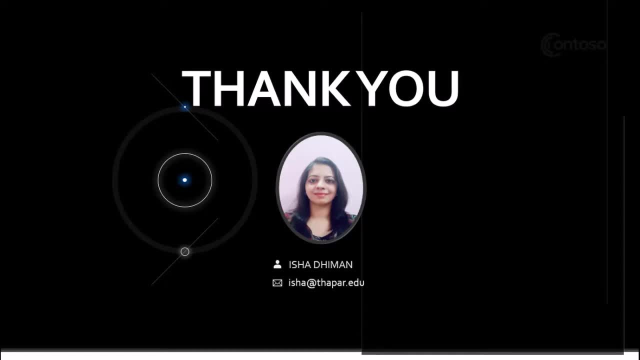 progress in the project. so that may be near to mst or after mst. so rest of the things will be clear when we'll actually be moving into the course. so that's all from my side. thank you, uh. this is my email id, isha, at appleedu, so for any queries you can contact me at this email id. you.